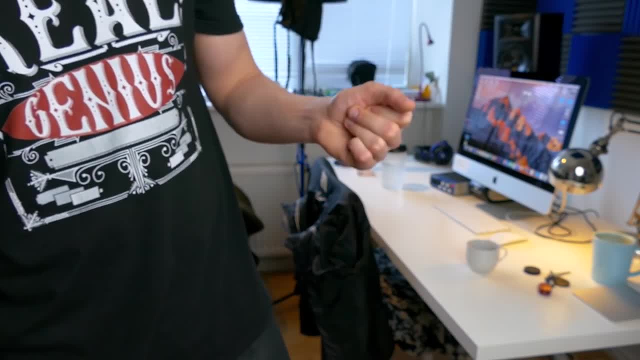 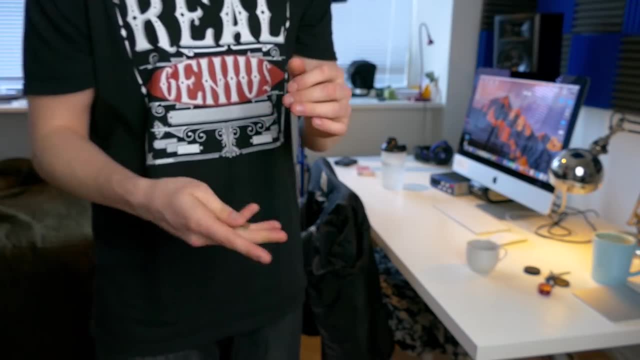 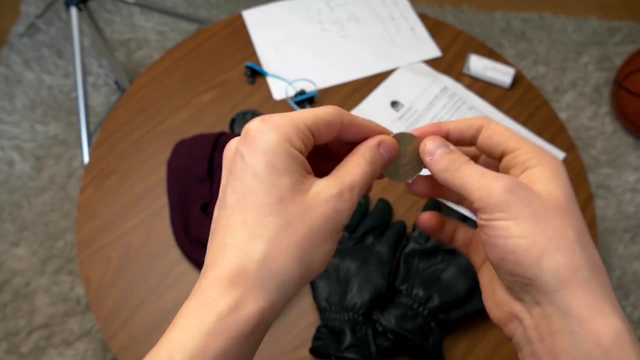 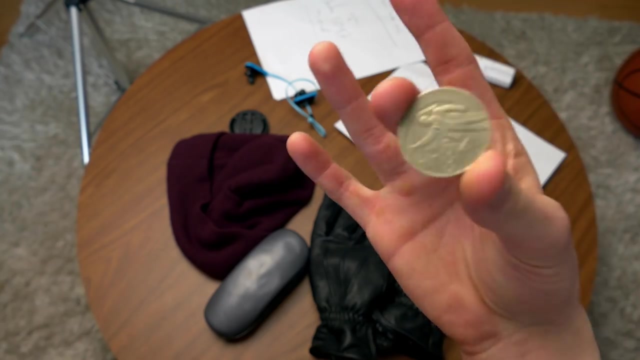 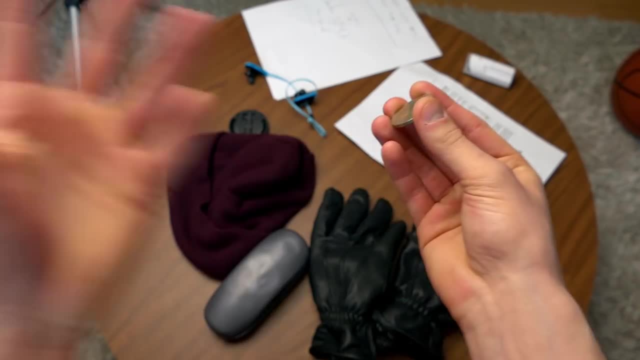 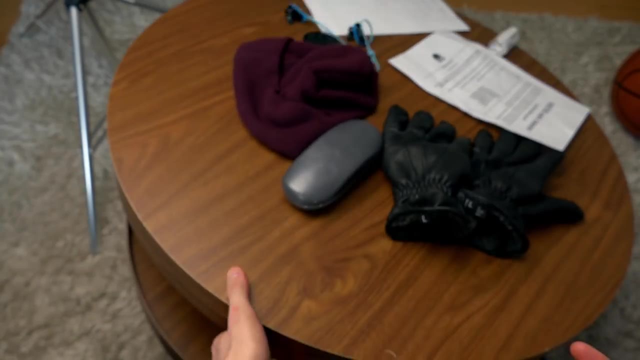 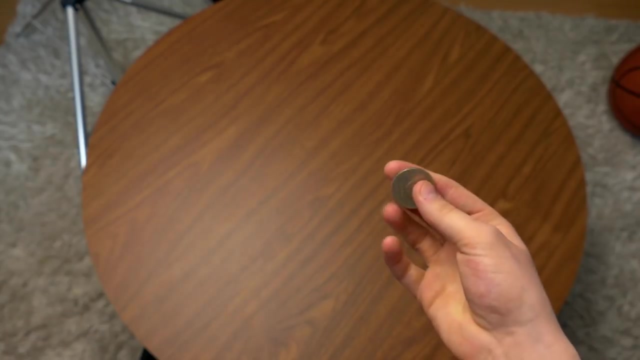 your other fingers, they can also hold the coin for support. so it's a little bit easier in the beginning. and, man, my table is so messy. wait, just like that. now it looks nice and clean and professional, right, boom. so you're going to be holding the coin like this. but if this move is 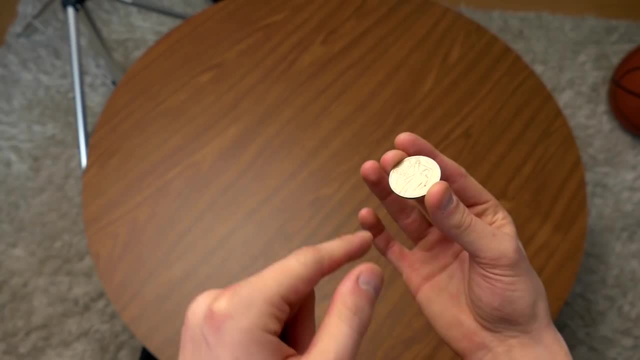 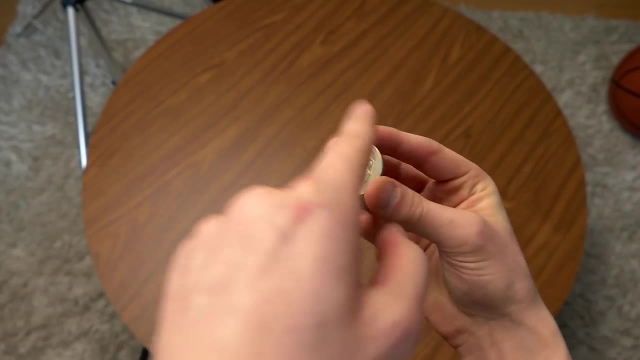 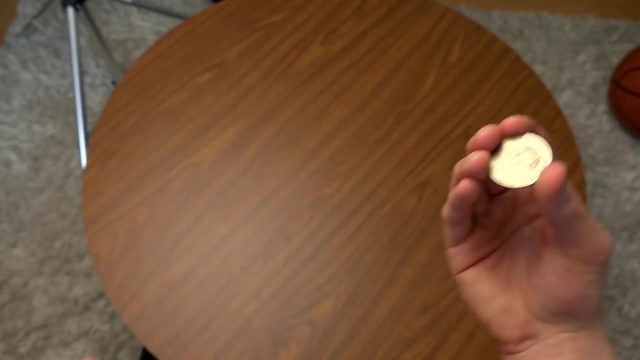 really difficult for you, then i would recommend starting off practicing this move by holding the coin with these three fingers, so your index, middle and ring finger, because then it's going to be easier to do in the end. so once again, it looks something like this and it disappears, and then 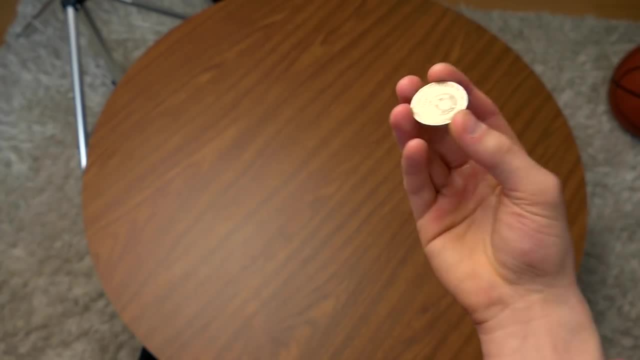 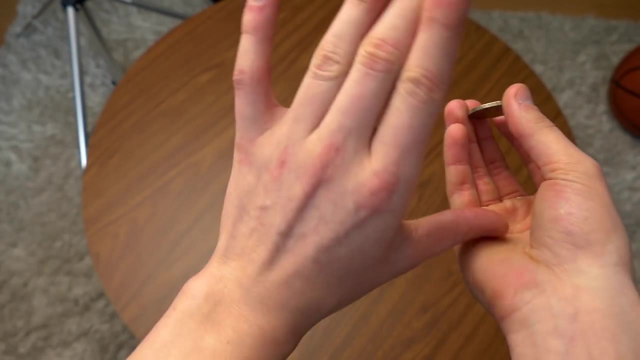 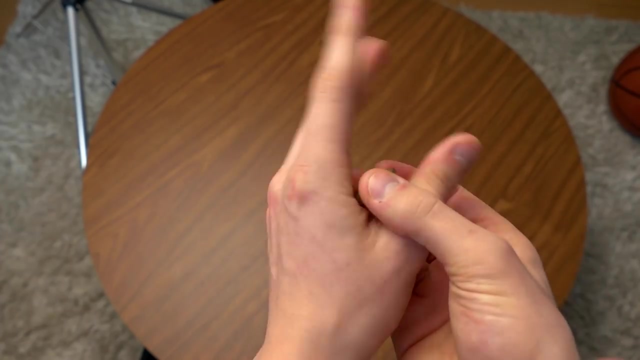 it's in this hand. so here is how this is: once you are holding the coin, your other hand is going to come by just like this and, as you can see, your thumb is going to be beneath the coin and日本, And in the action of trying to take the coin, then you're going to drop the coin down. 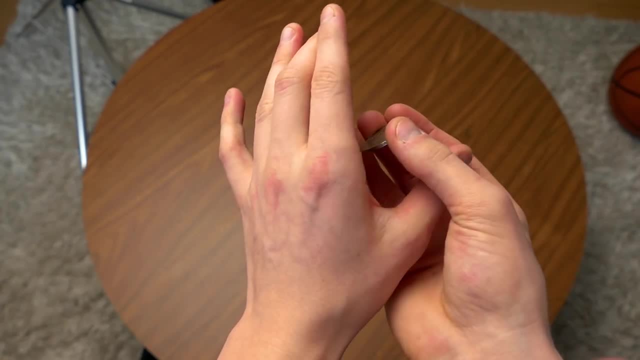 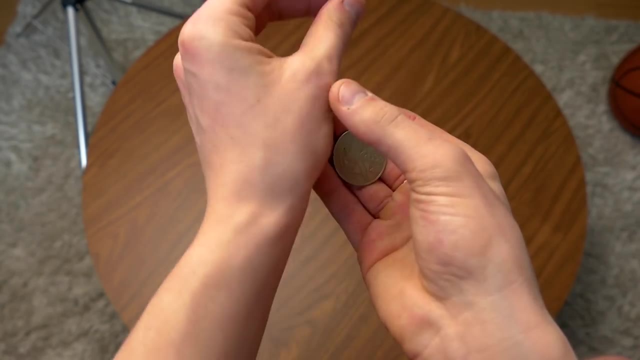 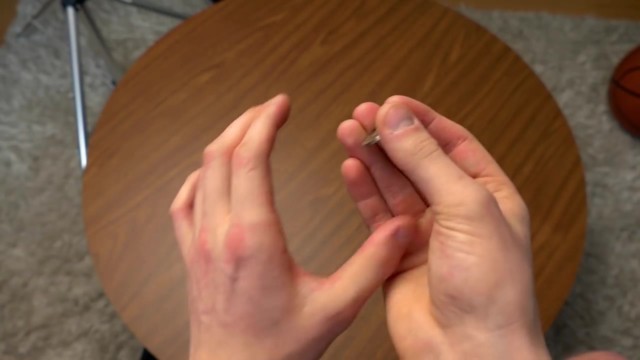 So here's what I mean Basically: you do this and then you drop the coin just like that, And now there is space, as you can see, for the hand to come through, Because if the coin was here, then your hand cannot go there, And when it drops, then you go and act like you take the coin. 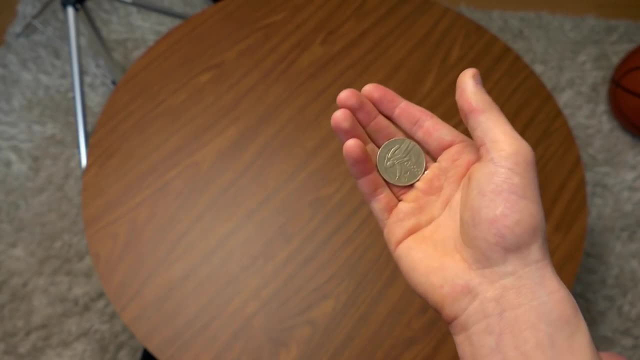 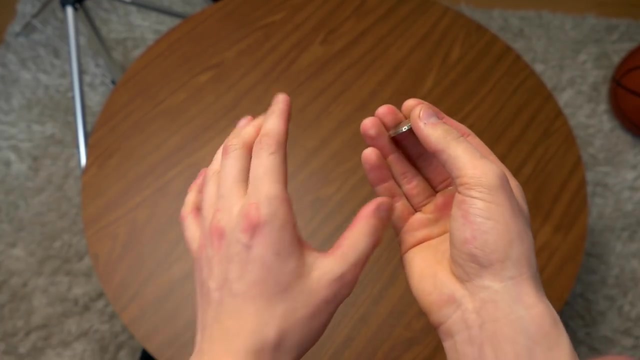 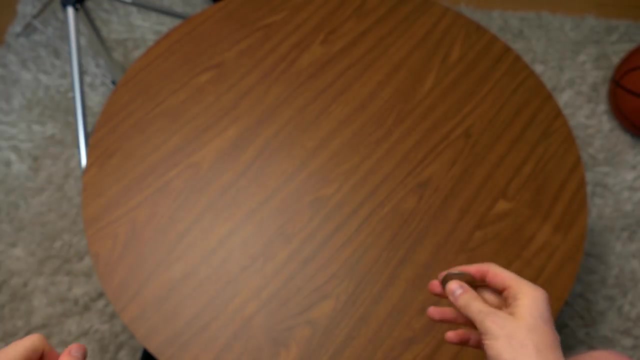 And this hand a lot of people. they have a few different discussions about this hand and what this hand is supposed to do. Some people they say, well, just hold your hand close to your body for a few seconds and then drop it down. But in my opinion, it's more natural to do this. 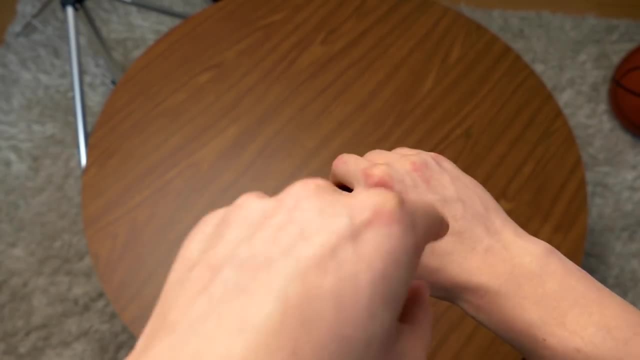 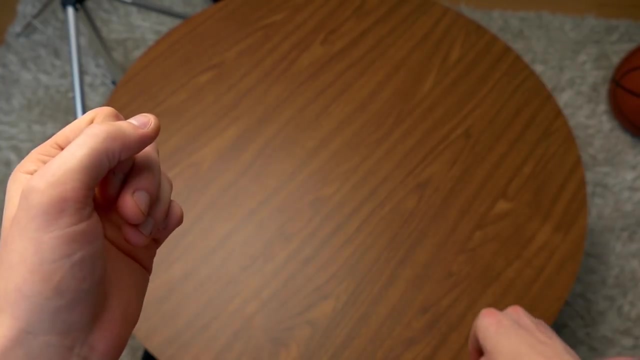 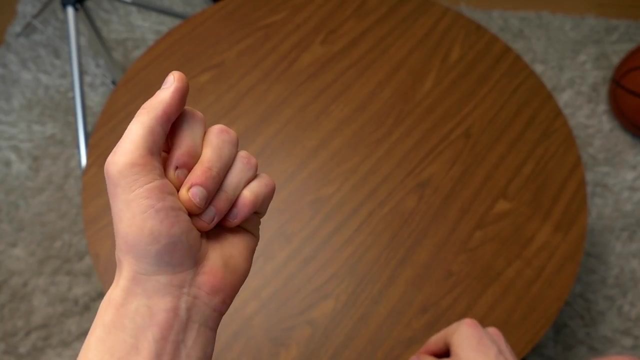 Just quickly drop the hand down. So, as you can see, look at this hand, at my right hand, So my right hand- it quickly drops down. You know not like this, But it drops down in a natural speed. if this makes any sense, which I hope it does, 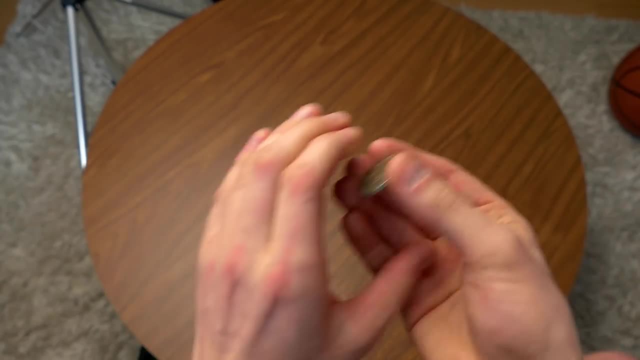 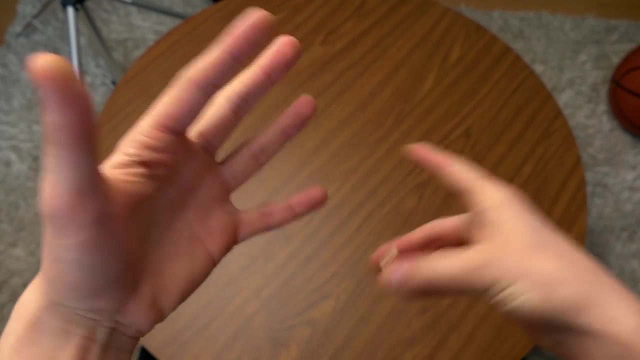 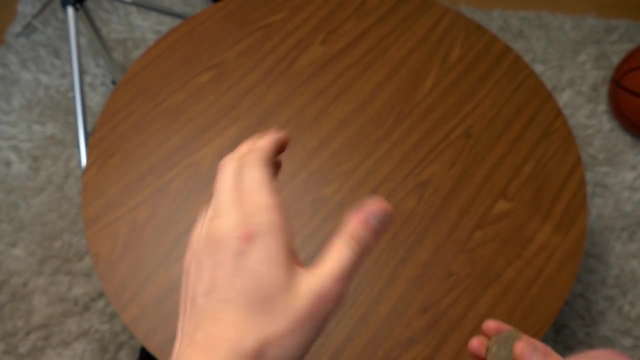 Your thumb comes here and you also cover the coin by using these fingers. So make sure that there are no windows, which means no gaps in the fingers. So try to act like you take the coin, Act like you are palming the coin, so no one can see through the fingertips. 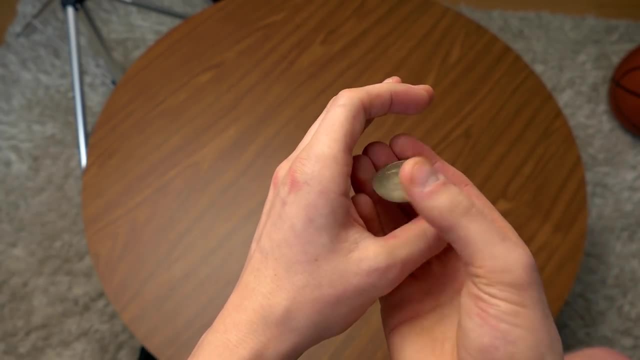 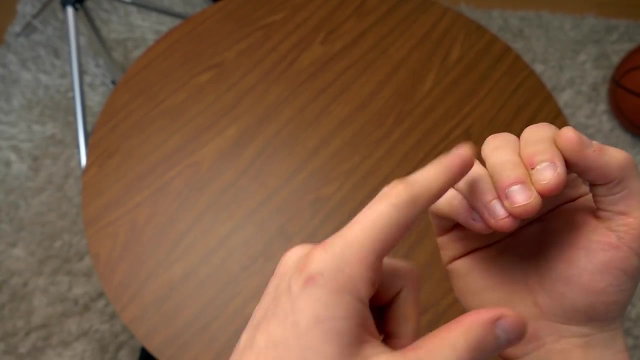 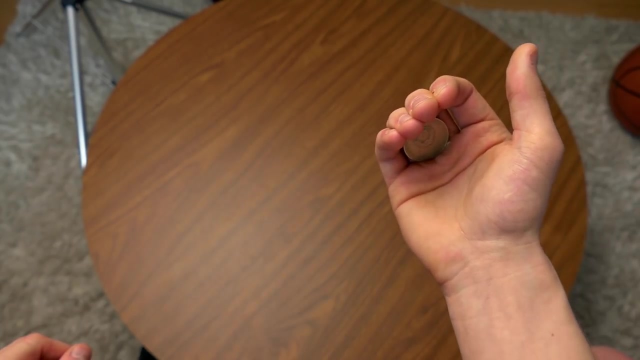 And then, once you have covered it, you're gonna drop the coin and then you're gonna act like you take it Now- this can take a long time to learn- And also use these fingers to cover the coin from the spectators eye level, And if you want to do it surrounded, then just do this. 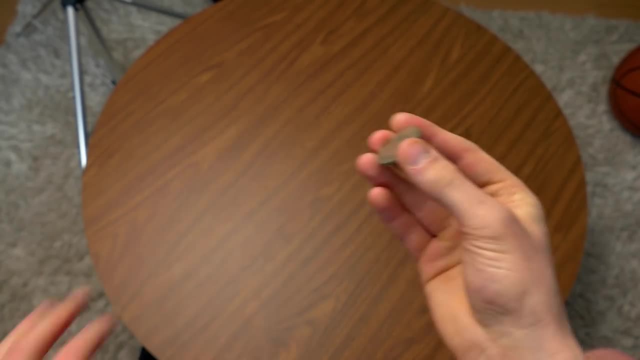 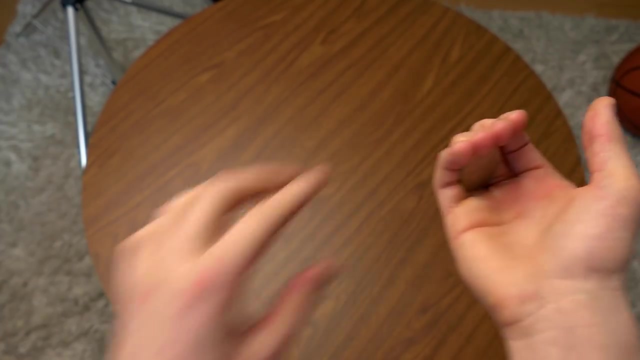 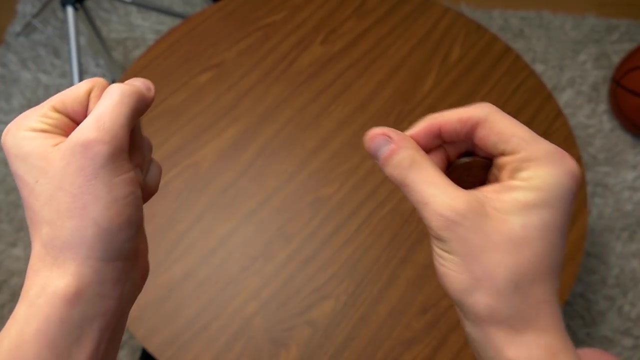 Because then no one can see anything. So, basically, if you do it in front of spectators, then just do this and hold the hand like this, where the fingers they're covering for the coin, And if you're doing it surrounded, then just do this. So instead of holding the hand like this, then you squeeze it and hold it. you know, you know. 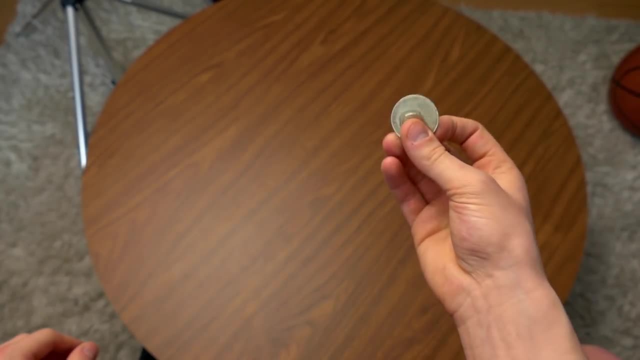 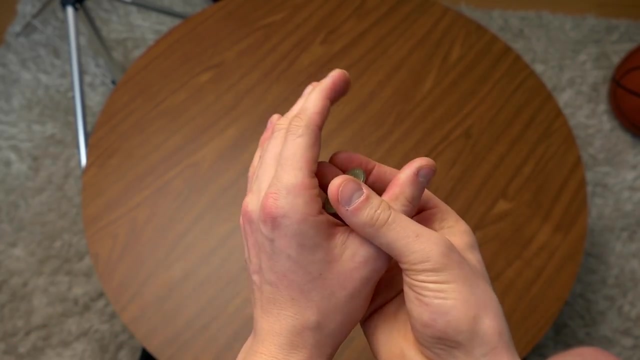 like this: All right, Man, I'm so disgusting sometimes. So, yes, that's how you do it Basically. you hold it Right there And then boom, you act like you take it, And then you tell the spectator: look, I have the coin. 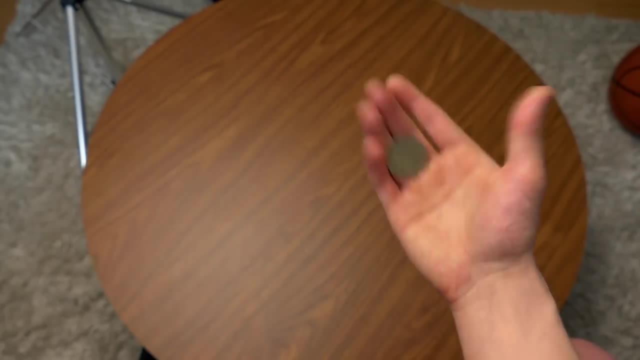 If you blow on it just like that, it disappears And then it's in this hand. All right, Quite easy to do. Also, when you feel like you can do this move, good enough, then try to hold it just with these two fingers. So try to hold it like this with the two fingers.